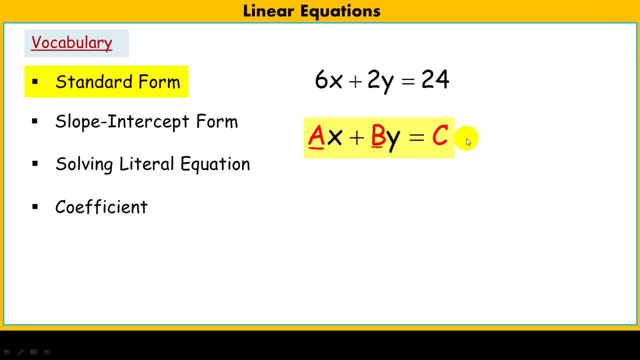 And this is considered standard form and this is really really useful, particularly when we want to find our x and y intercepts. But when we want to graph, slope-intercept form is a really handy way to do that. This is kind of a function. 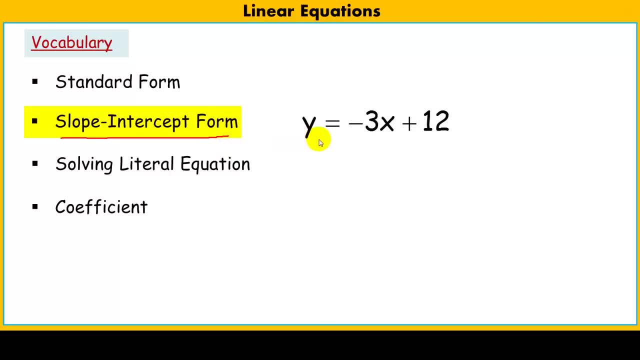 This is a function form, because we're going to get y alone, And this is what it would look like a typical linear equation in slope-intercept form. Notice: now I have y alone, I have a variable term in x with this coefficient of negative 3 and a constant hanging out here. 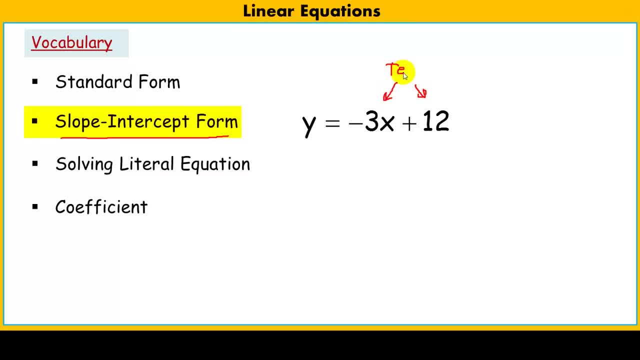 Notice there are just two terms And I have- y is always alone over here, In slope-intercept form, these particular things. the coefficient negative 3 is considered the slope of this line- And we'll talk about slope in another lesson- And this number, this constant here represents the y-intercept, or where the line crosses the y-axis. 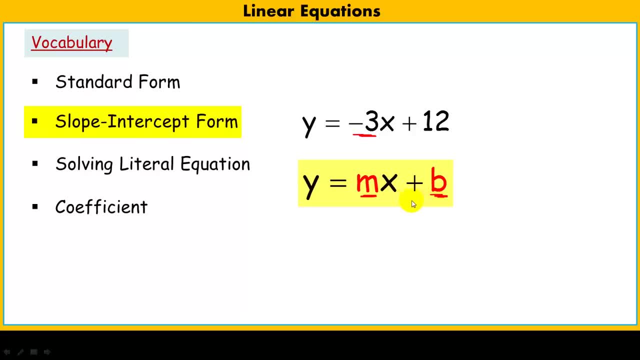 And again it has meaning. So the big deal for us in converting it to slope-intercept form is we have it in this exact form. In other words, we want to get this variable term in x Separate from the constant over here. 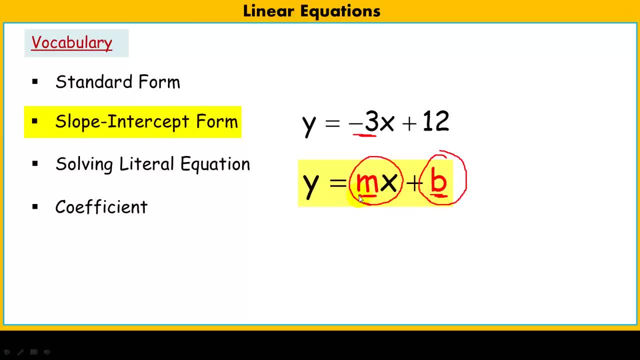 And we want to have it in two terms And we want to be very clear as to exactly what our coefficient is. So we will be using the idea of solving literal equations, That's, an equation that has more than one variable in it And obviously, you see, this is a literal equation. 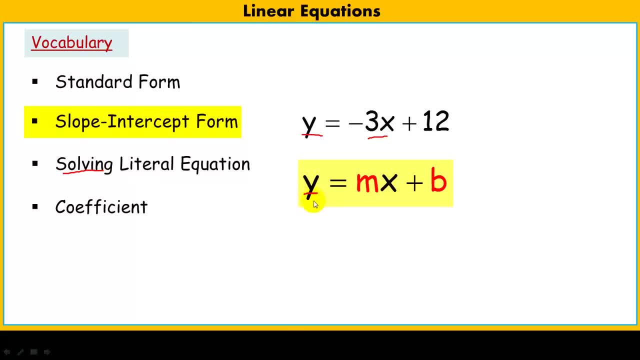 And what we're going to do is we're going to solve for y. We're going to get y alone And coefficient. again, It's very important that you understand what a coefficient is. It's that number that multiplies a variable. So in this case, m, the coefficient for x, is going to be our slope in this. 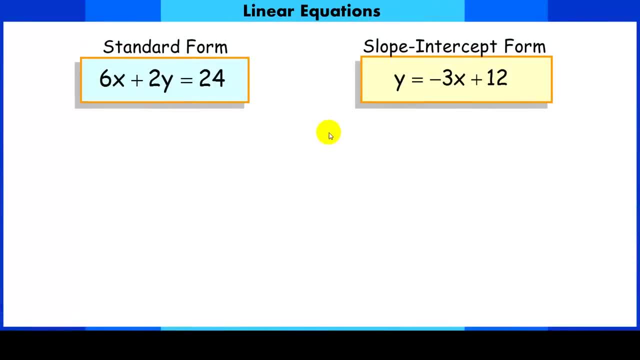 And again, we'll talk about slope in a later lesson. All right, Well, the two example equations I used are actually equivalent equations. It's just one is a different form for the other, And I could really put an arrow going both ways. 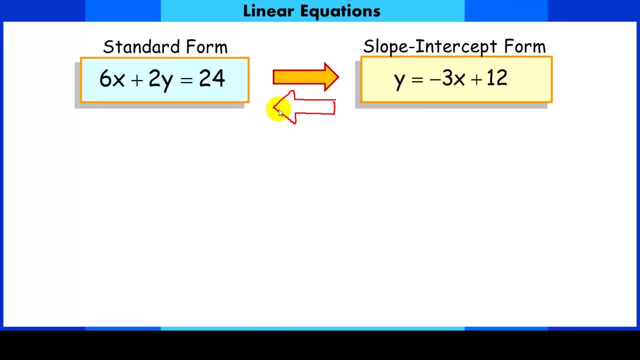 Because they are equivalent. This could be converted back to standard form if I wanted, But what we care about today is converting something from standard form into a slope intercept form by getting y alone. Okay, So to get y alone. So here's what we do. 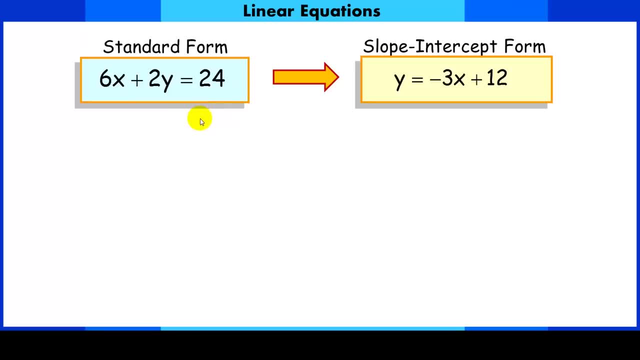 It's nothing entirely new for you guys, except for a little bit at the end. So the first thing we want to do to get y alone- Notice I've highlighted y- We're going to subtract 6x from both sides. Now, normally, or what we've done before, is when we subtract the 6x. you would have seen something like this: 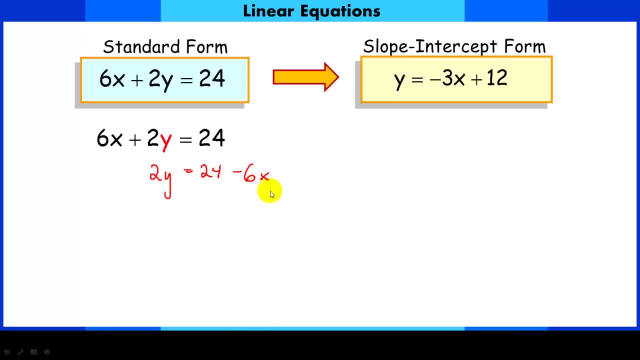 Equals 24 minus 6x. But we don't really like it like this, because I want to have my variable term in front of my constant. So what I'm going to do, I'm just going to move him over And then, when I subtract 6x, 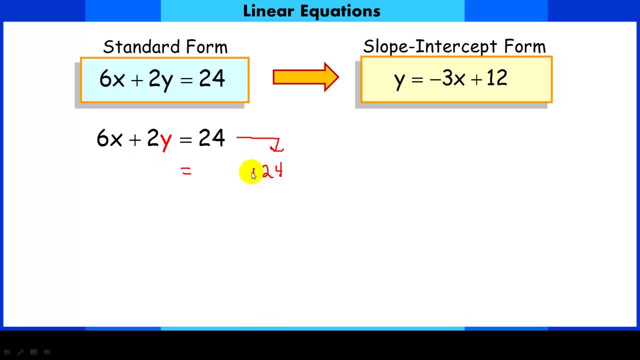 From both sides. I'll have my 24 over here, but then I'll have my negative 6, 6x here. commuter to property- because we are just adding these two terms means I can do it in any order, And this is the order I want to do it. 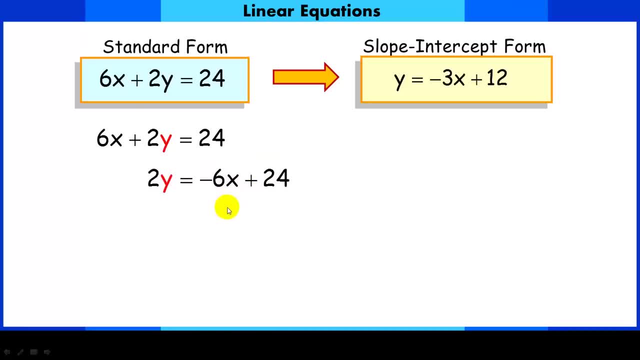 I want to have my variable term in front Now. once I get that, to get y alone, we're going to divide by two. Now, before we've done something like this, we divide this whole side by two, which is entirely algebraically correct. 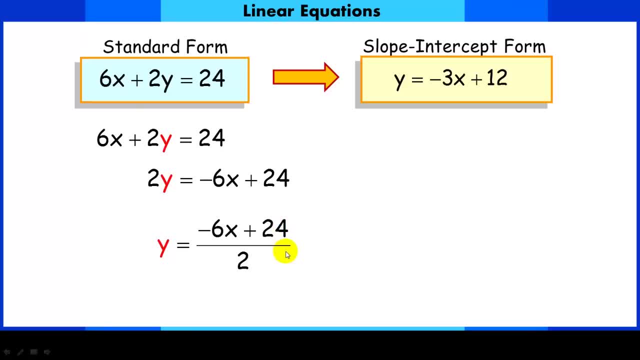 And before this would have been our perfectly fine answer. However, now we want it in slope intercept form, So I want this to be two terms. So what we're going to do is like when we came over here and divided by two. really, since we're dividing this whole thing by two, in a way, we're supposed to be dividing every term by two. 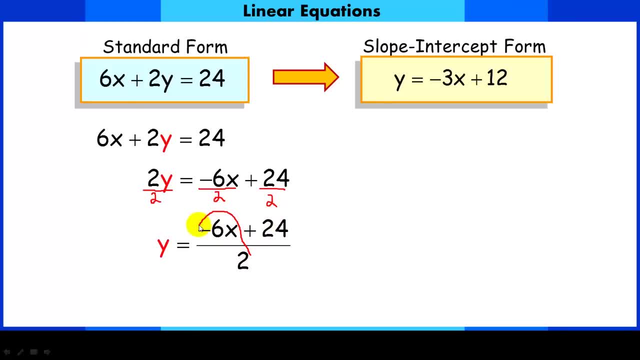 In other words, this negative 6x is being divided by two, but also 24 is being divided by two. So it will look something like this: Now, in each term we would just simplify: Negative 6 over 2, well, that would just be a negative 3.. 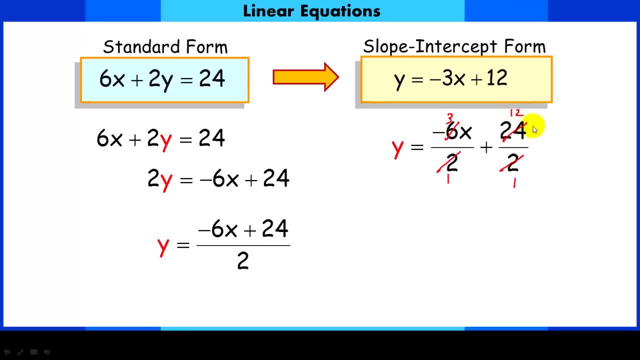 24 over 2,. well, of course, that's just 12.. And that's how we get our forms the same. So this new form, this would be considered the linear equation in slope intercept form. Okay, so let's try a couple. 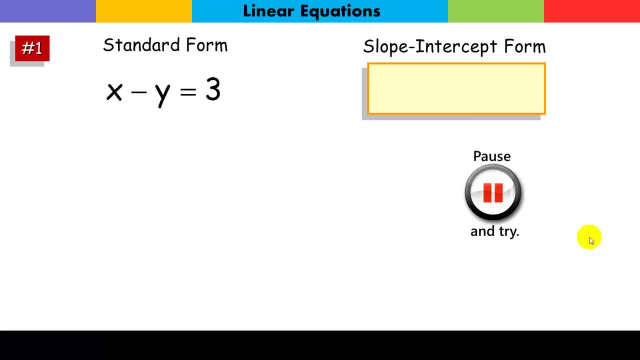 Okay, Take a second. Take a second and go ahead and convert that x minus y equals 3 into slope intercept form. Okay, again, we want to get y alone, So I have to get everything else on the other side and I have to have a certain sequence for that. 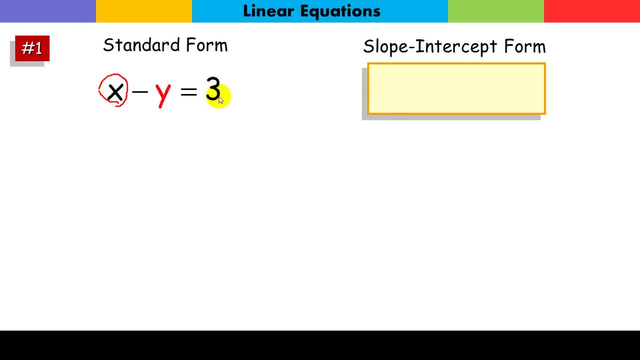 So the first thing I'm going to do is I'm going to subtract this x off of both sides, But remember, I'm going to move this guy over because what I want to do is have the variable term in front of the constant, So notice. 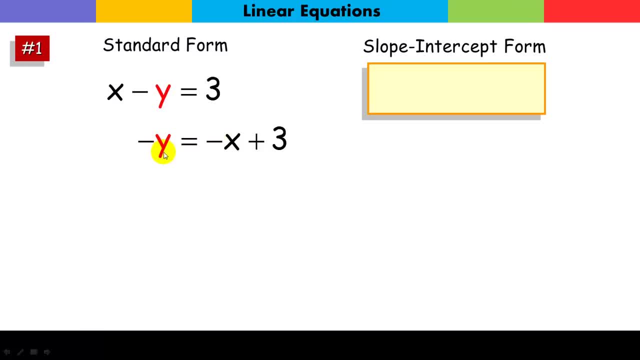 I just scooched him over and subtracted x from both sides. But y is not alone right now. Right now we have a negative 1y, So if I want to get it alone, I'm going to have to divide by negative 1.. 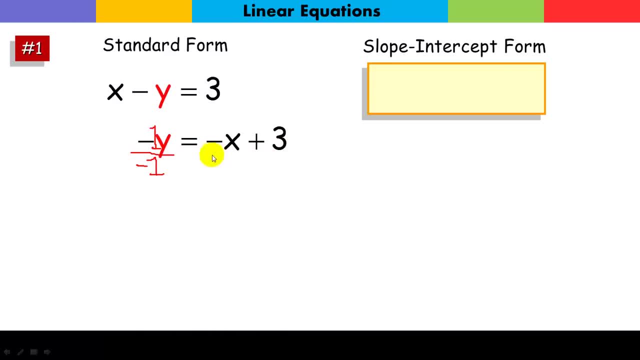 And if I divide this side by negative 1, I divide this whole side by negative 1, which means every term by negative 1.. When we do that now, I am going to get y alone, Negative x over. negative 1 is just a positive x. 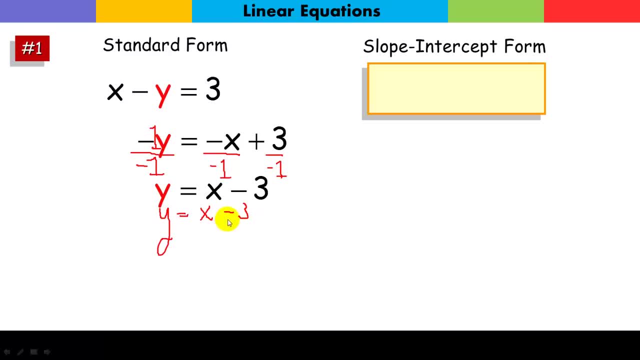 3 divided by negative 1 is a negative 3.. And now I can go ahead and remember. the coefficient for x is 1.. Sorry about that slide. Okay, Let's try the next one. Go for it. Okay. So we want to get again. we're looking to get y alone. 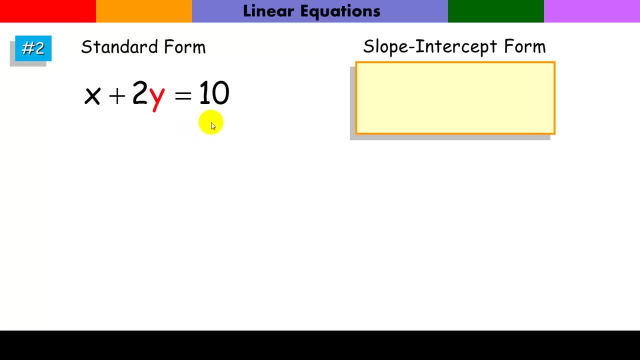 And, like before, we've got to subtract x from both sides. And, just like before, I'm going to scooch this guy over to make room for my Negative x. Now I'm going to divide each term by a positive 2.. 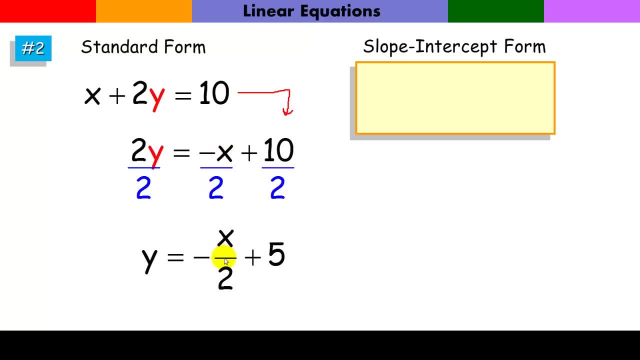 And so, of course, I would get y alone. I'd have negative x over 2 plus 5.. Now one thing: there's a problem here. Some students would have a hard time understanding what the coefficient is on this. Well, understand that a negative x over 2 is the exact same thing as negative 1 over 2 times x. 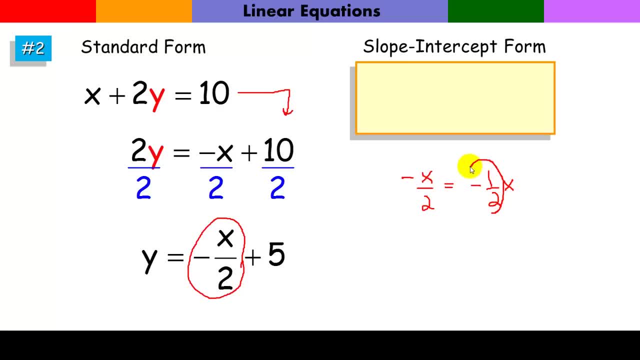 Okay. So really, in this situation we want to express any sort of fraction like this, Because then we know very specifically what the coefficient is. And remember, the coefficient is important because that represents our slope. So the correct way to write this in slope intercept form is: y equals negative 1 over 2, x plus 5..